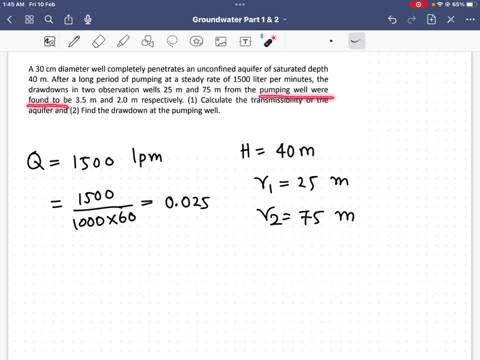 pumping well were found to be 3.5 meter. so that's mean this will be my s1. so s1 will be 3.5, s2 will be 2.0, then i will i. now i have to find out the transmissibility. all right, so for this one, this is the. 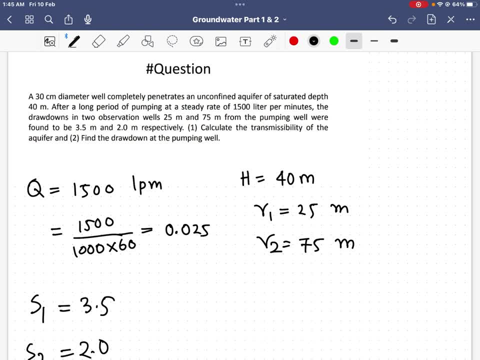 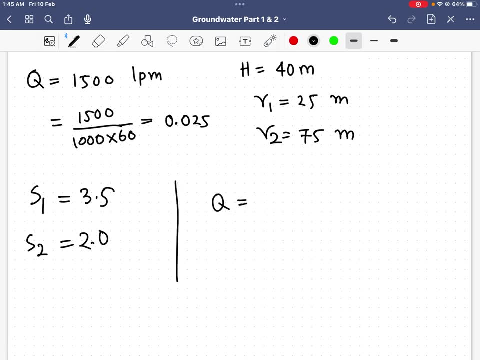 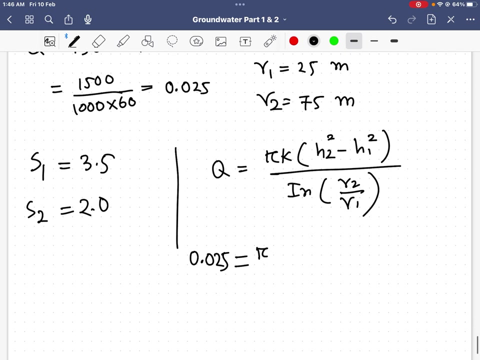 unconfined aquifer. so we have to apply the different formula and the formula is: q equal pi, k, h2 square minus h1 square divided ln, r2 divided r1. all right, so i have my q, q already, i got it. 0.025 then pi. i don't know the value for the k. 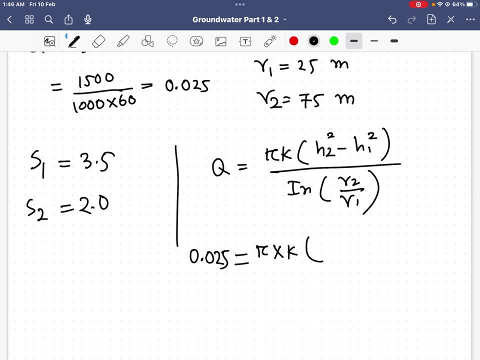 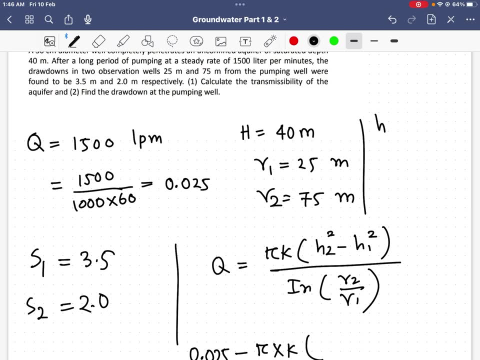 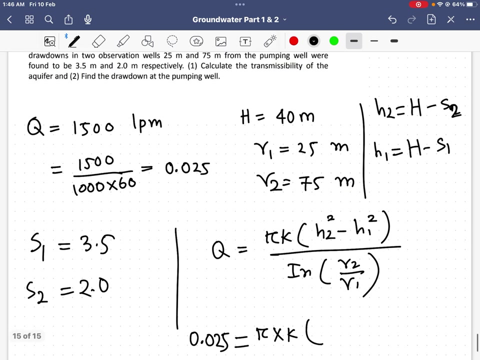 i will find out this k by using this formula. so i have this h2. okay, how i will get the h2? i will get the h2 from this formula: h2 equal the length, h minus s1 and h1 equal. okay, h2, sorry, and h minus s1. so my h is 40. so if i subtract s2, value 2, so i 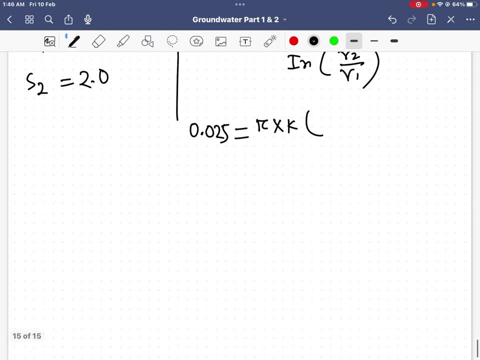 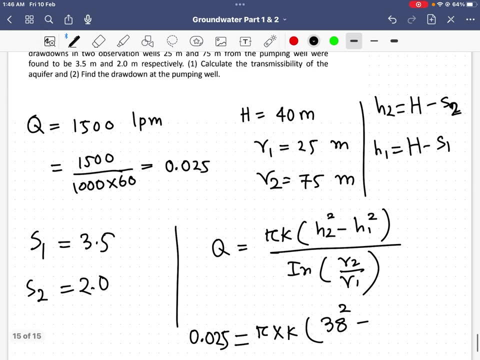 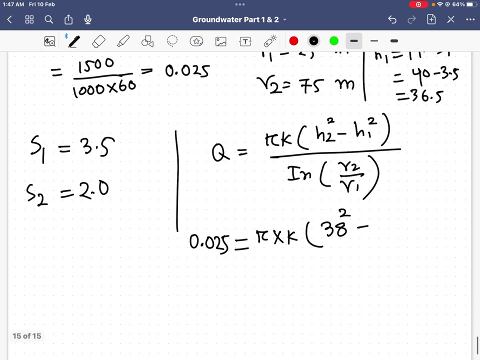 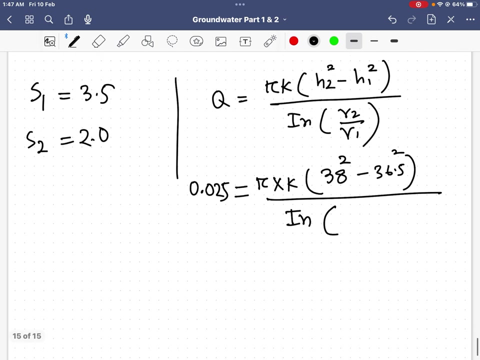 will get 38, so i will get 38 for h2. so i will write 38 square. and for the h1, my h value is 40. i subtract s1 value 3.5 from here, okay, will get 36.5, so 36.5. i have to square divide it long: r2. i have this r2 75 divided 25, my r1. 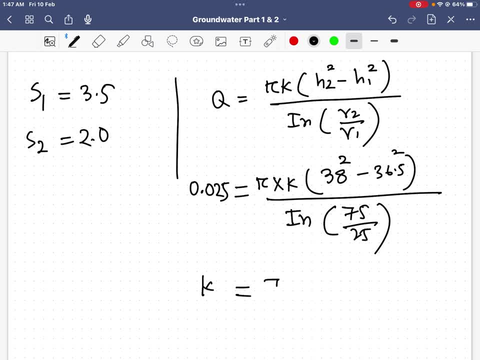 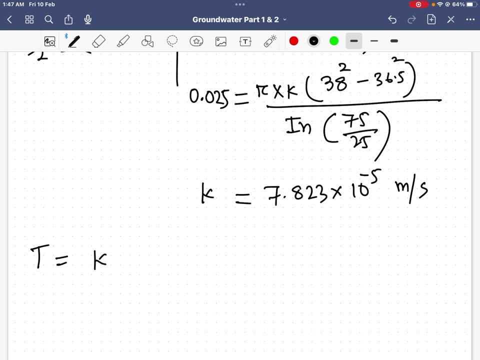 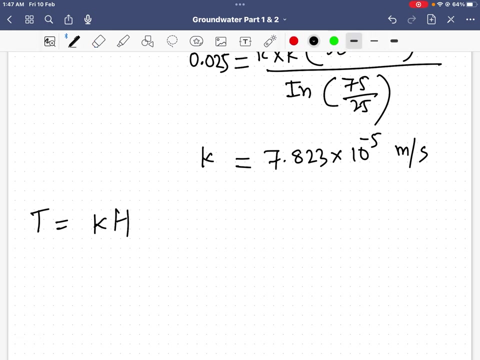 if i calculate, i will get my k. my k will be 7.823 times 10, power negative 5, and my k permeability will be in meter per second. once i get the k easily, i can get the t, because i have to multiply only k and b, so in this case it will be height. so i will put h and k. i already got. 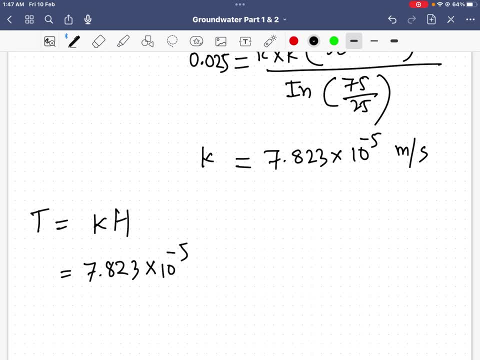 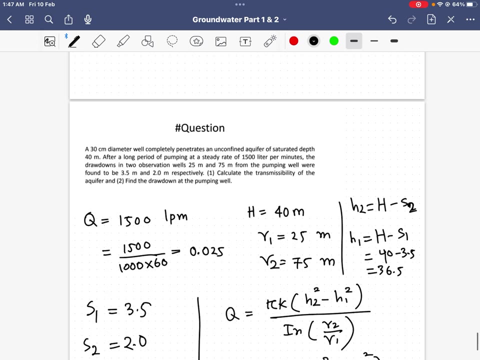 7.283 times 10 power negative 5 times. i have the h. h is my 40 meter, so if i calculate i will get 3.13 times 10 power negative 3. this is my transmissibility. all right, so i already find out this transmissibility. 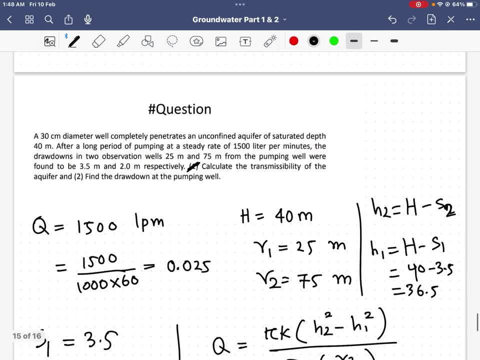 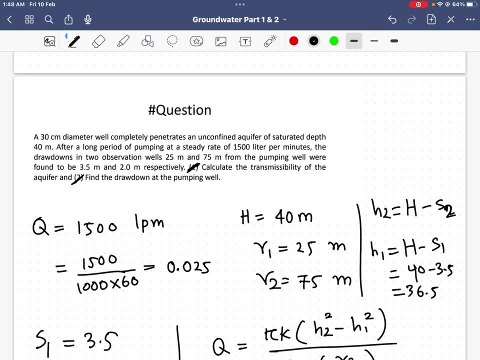 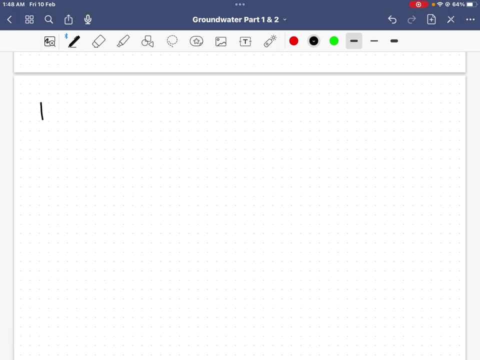 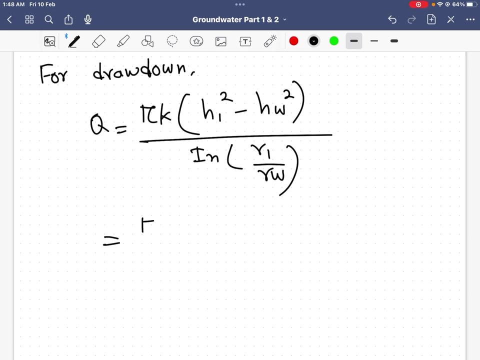 so now i will go for the second questions. okay, find the drawdown at the pumping. well, so for find out these questions, i will solve through one formula that we already know for drawdown: q equal pi, k, h1 square minus hw, square divided lone, r1 divided rw. okay, so from this formula, i will 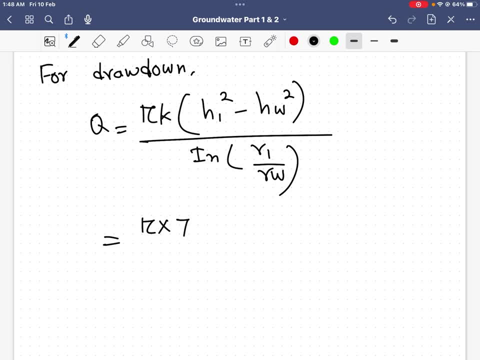 get pi. i have this k already. i find out from the previous solutions: seven point two, three, ten point, five times. okay, if i have the h1, i know that my h1 is 3.5 times. i know that h1, i know it. fifth, and отвечer y equal pa. I plan to solve this problem. or, if i have the a times a, try and solve this problem, or in end now I have done one question b plus bсл. I said that 7.23 times 10.5 is plus x, as. a primary value or in the clients of that. so I have divided the k by 16 and this is not going to be next enough so that I will do the final answer: k minus a by 16. so this result: I do not need to do a. 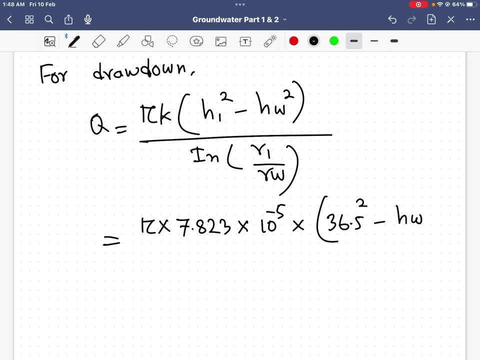 traditional these 1.3 to 0. now I have this pst, so we get my p1. we have to do pi as volume rate of bringing 3.5 square minus. i don't know my hw square because this is my drawdown. okay, divided long. 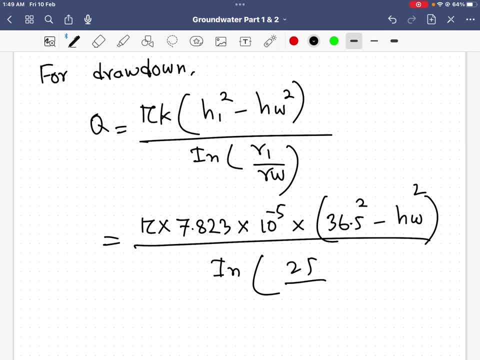 i know the r1, so my r1 is 25 and rw 1.5. because how i get? because 35 centimeter diameter, so from there i can get my rw. so this is the way to get: rw equal d by 2. so my d is 30 divided by 2. so 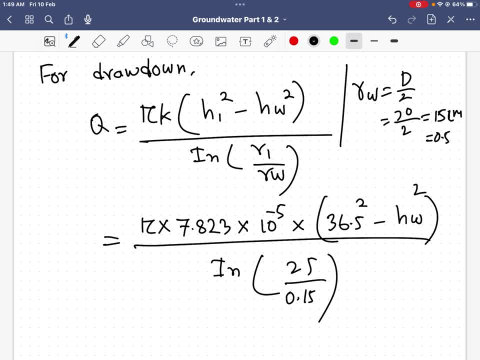 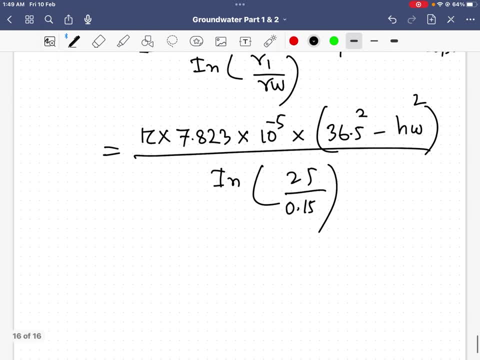 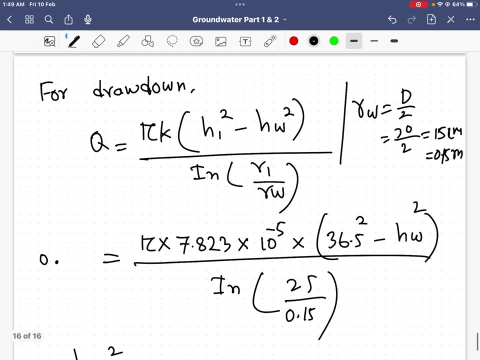 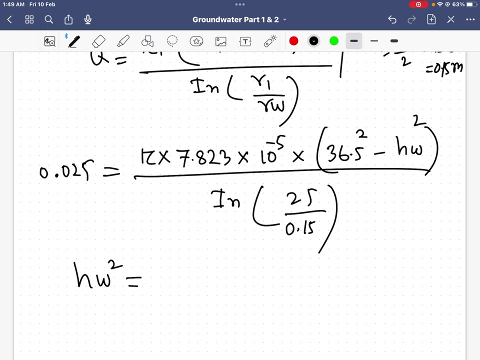 15 meter centimeter, so i have to make it meter, so 1.0.115 meter. so if i calculate here, so i will get hw square, because my q is 0.. my q was 0.025. okay, 0.025, then i will get 81.80, 811.80.